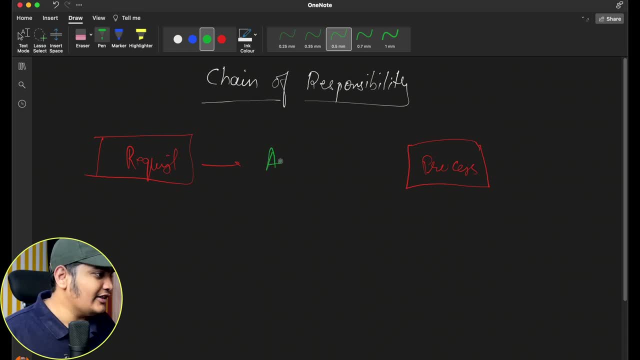 for the ordering system. those are properly authenticated. So you add the authentication part as well. between the order processing and the request that comes in: Okay. so after sometimes you also add that: okay, whatever the process is coming, that also has to be. 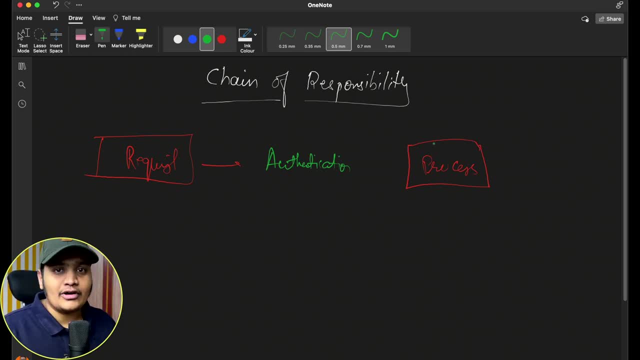 properly authorized. So a proper request has a proper authentication, proper authorization or not. is a request by a customer or is request by admin or not? that you have to identify and accordingly you have to do some processing on it. Okay, so you add the authorization. 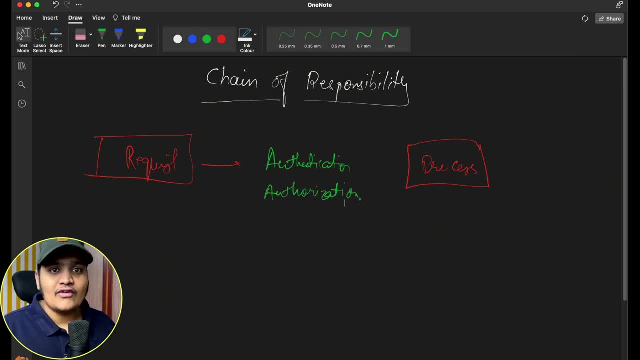 as well. After that- after sometimes, you get a new requirement to add some of the validation as well. So you go ahead and add some validations And after that your system is really working well and you're getting a lot of orders to get processed. So what you try to do is you: 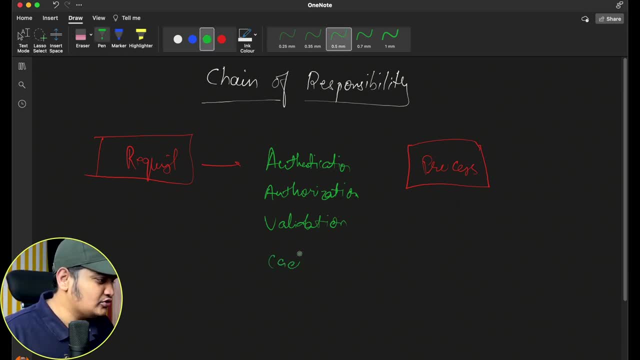 add a caching system as well. So suppose you're adding a caching to this particular system and you're adding a bunch of more different things just before processing your order. Okay, so you can see that this is a lot of details that you are adding here. 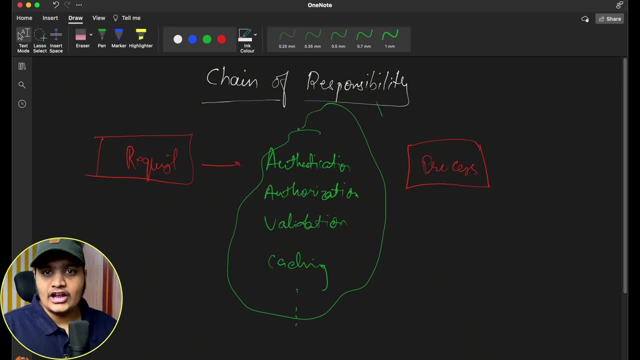 just before doing the processing, Just to process your order, you're adding a lot of different things right, And sometimes that also happens, that some of the validations or some of the processes you don't need as well. So suppose sometimes you don't need. 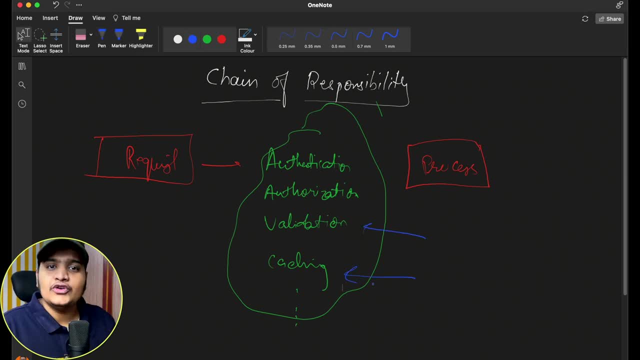 validation, suppose sometimes you don't need caching as well, but still you do those cachings and validations and all those stuff and a bunch of other details, details or other processes that you have added in between the actual processing of the order. So you can see that this type of scenarios occurs very frequently as well. 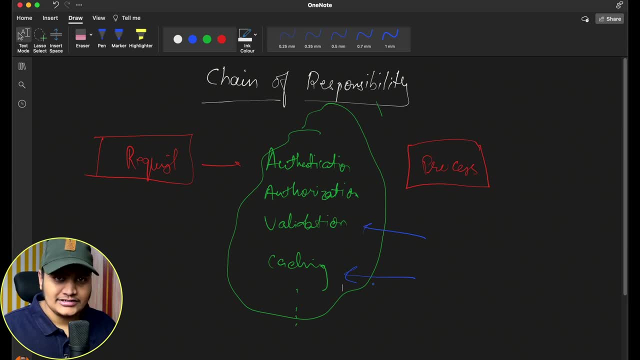 So to avoid this problem and to avoid unnecessary calls, what we can do is we can add the chain of responsibility design pattern. What chain of responsibility design pattern will do is it will have a appropriate task for doing appropriate things. It will have authentication, will have just to do authentication and after authentication. 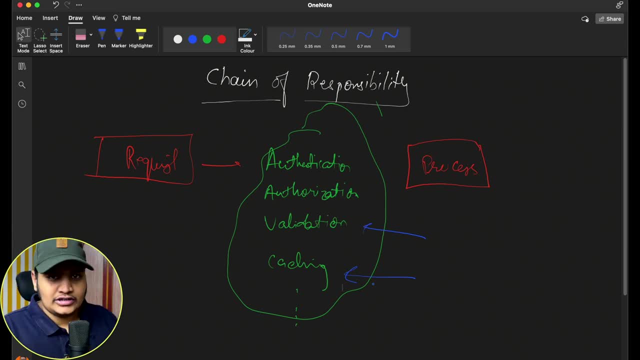 you can tell okay, once the authentication is done, you can move to authorization. So you can see that you are passing the request and a data from one responsibility to the other responsibility. Once the authentication is done, and if the user is customer, then you have to do some. 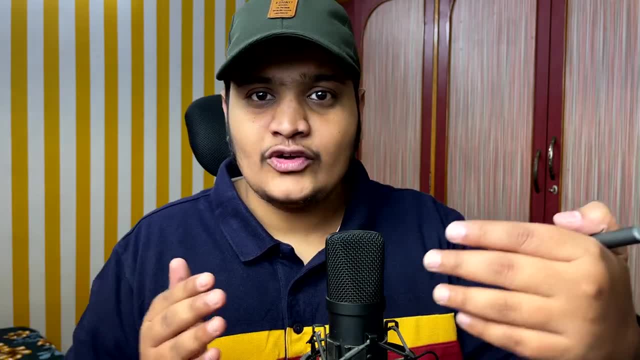 other stuffs. If the user is admin, then you have to do some other stuffs. So you can see that there is a bifurcation there, but there are other stuffs you need to do, right? So, based on that, based on some conditions or based on the 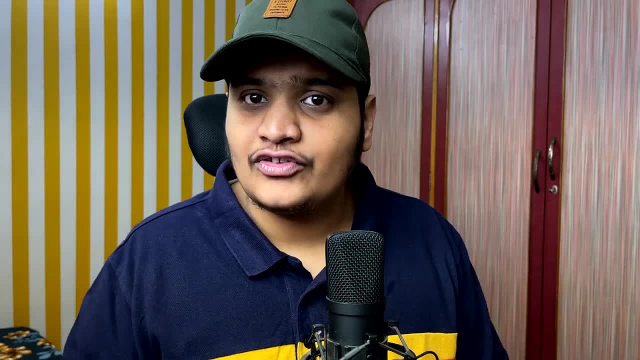 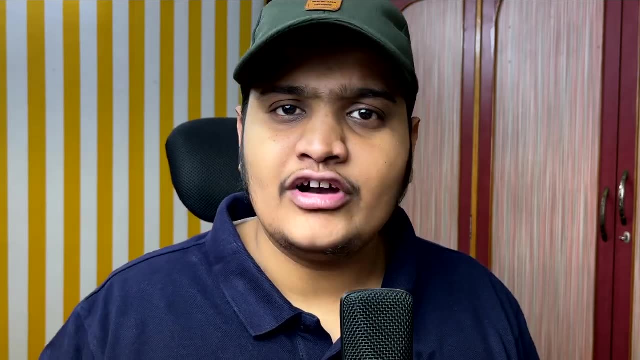 some logic. what you can do is you can again process those different conditions, different responsibilities, right? If it's a customer, there is a different responsibilities needs to be done. If it's an admin, there is a different responsibilities that you need to done. 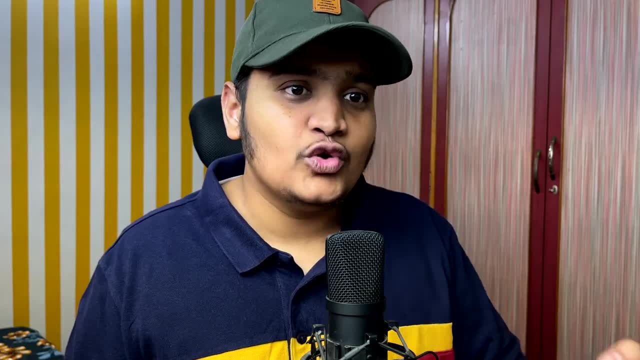 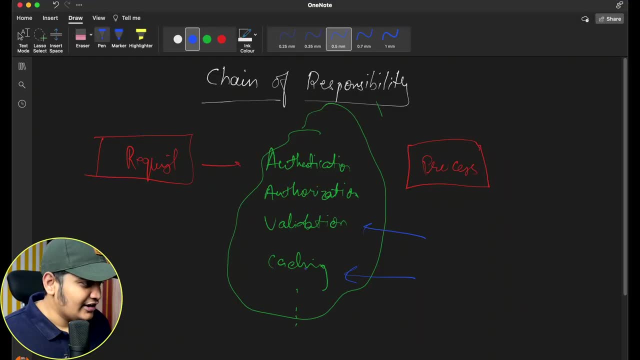 So with that, what you can do is you can define different responsibilities and those different responsibilities will be passed along the request and those operations will be performed. Okay, Suppose your caching is not required in admin, then you will skip the caching for the admin. 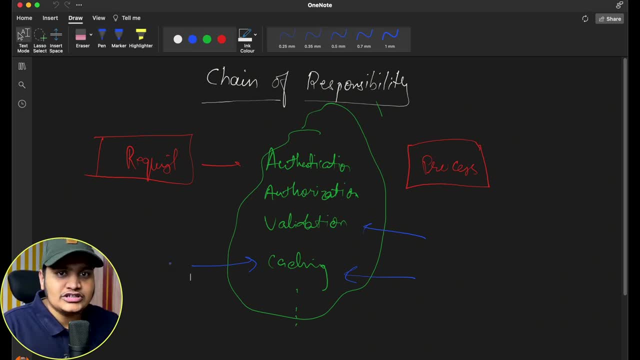 Okay, You will not pass that responsibility. The next responsibility that needs to be completed for the admin role, If it's a customer, yeah, caching is needed. So you will pass that caching as the next responsibility for the request. So you can see you are adding the responsibility, a chain of responsibility to be completed alongside. 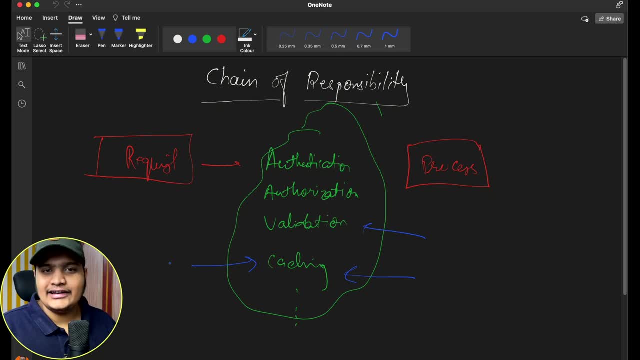 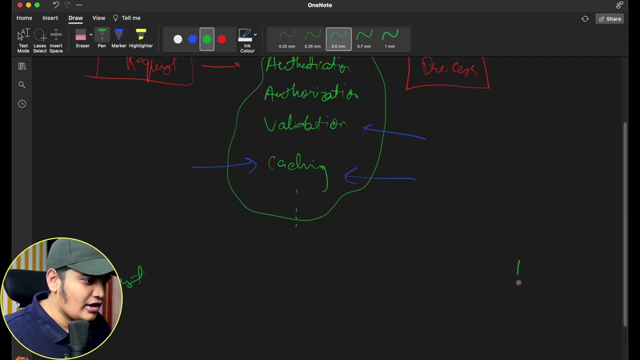 the request. Okay, So, because of this chain- this pattern is called as chain of responsibility- Okay, So, rather than doing this, what you will do is you will create a request, and this is your process, right? And what you will do in between is you will add a chain of responsibility. 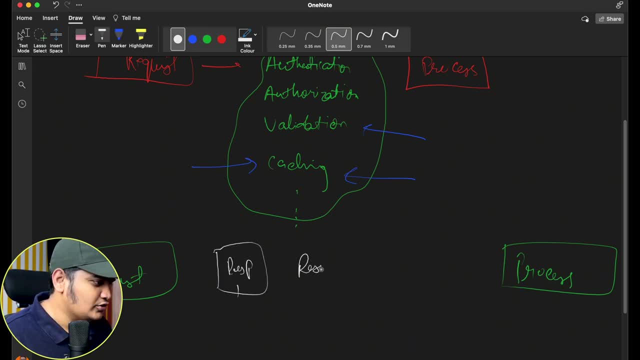 You will add responsibility one, responsibility two, responsibility three, responsibility four. Okay, All these responsibilities you will add And, alongside this request, you will pass all this data to all these responsibilities and whichever responsibility you're passing next, those responsibilities will be executed. 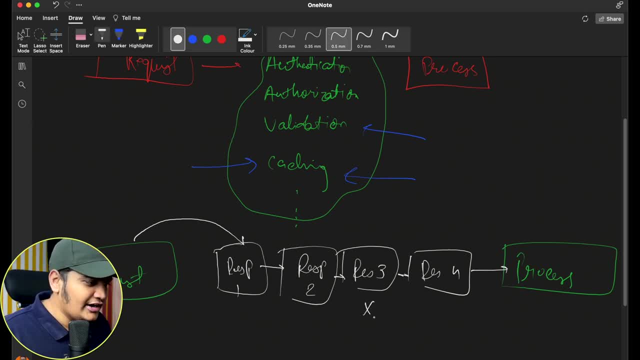 and your entire process will be completed. If some of the responsibility is not needed, you will can skip those responsibilities as well. Okay, So that's the general idea about the chain of responsibilities and pattern And where you can implement it now. to implement this, you will need an abstract class, which. 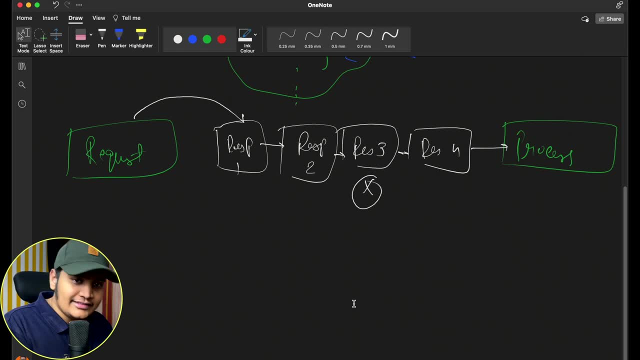 will have that particular responsibility and which will also take the next responsibility to be executed. Okay, So let's take the example. let's go to the code and see the example that we have taken up. What we have done is we have taken the example of a payment processing here. 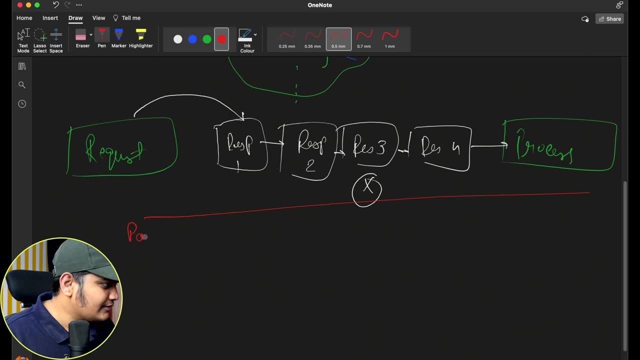 So I'll just give you the test here that we have the payment processing and we want to process some payments. Okay, That's a simple thing, And we have added a chain of responsibility. What we have done is We have different types of payment processing. 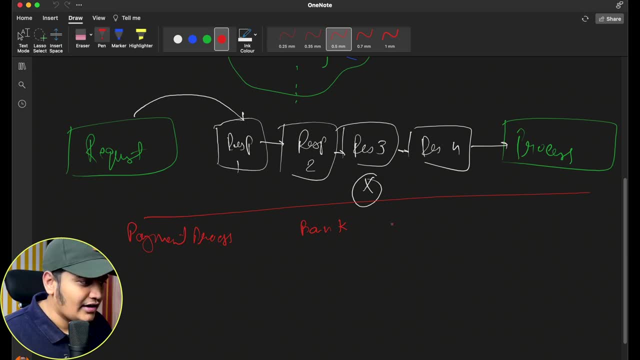 That is, the bank processing. Okay, You can process via bank. You can process via credit card, You can process via PayPal as well. This type of different processing you can do. Okay, And what we have added is that if the amount is less than 500, bank and processes process. 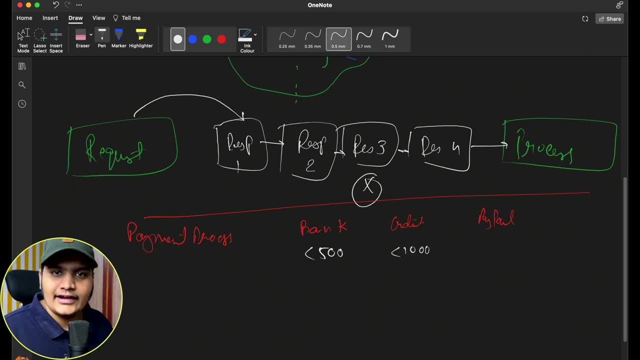 it. Okay. If the amount is less than thousand, credit card can process those payment, And if the amount is less than 1500, people can process it. Okay. And what we have done is We have added a chain of responsibility, Okay. 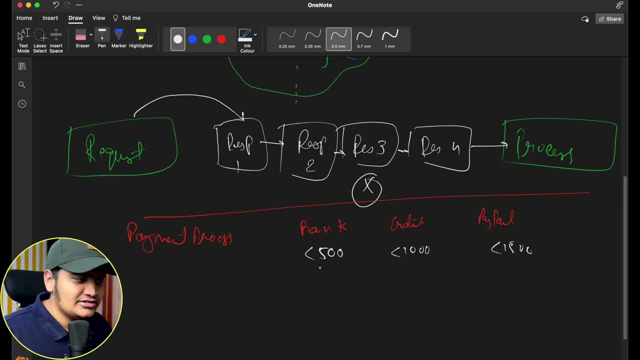 For a payment processor, for a bank, There is a responsibility that if it's not able to process this amount, it will add the next responsibility to the credit card. Okay, And if credit card is not able to process those payment, it has the next responsibility. 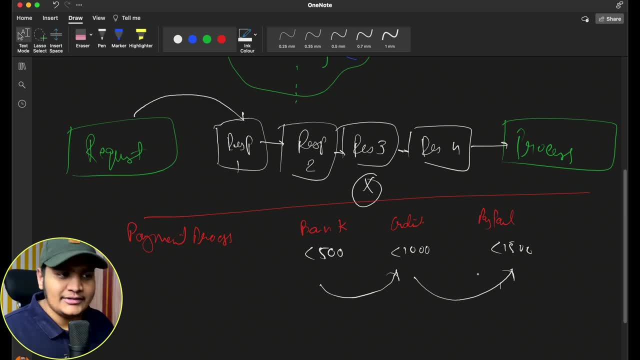 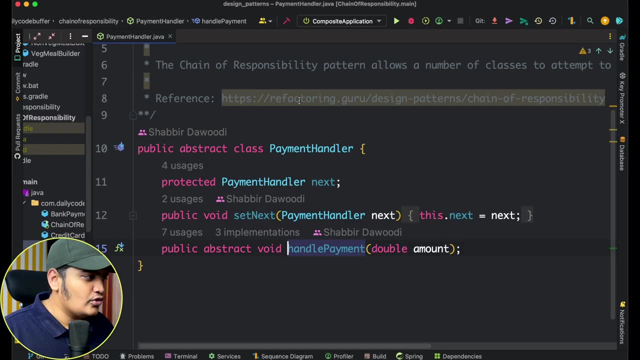 given to the people. Okay, That way the responsibilities are shared along and the payment will be done for us. Okay, So that's a simple agenda here. Let's go to the code, and here you can see that I have given the basic information here. 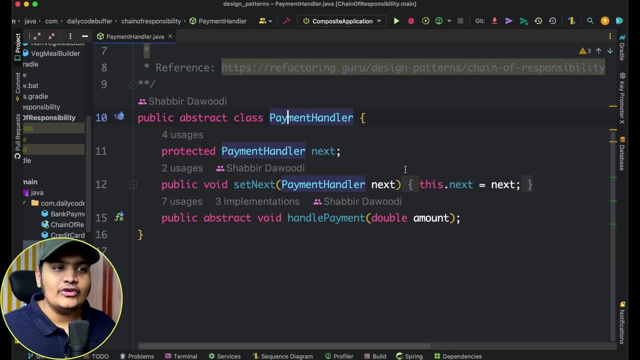 as well. I have also given from where I have taken this reference. So, if you want, you can go through this reference and you can learn more about it, Okay, And you can share some love as well to the creator. So now you can see, we have created a simple abstract class here. 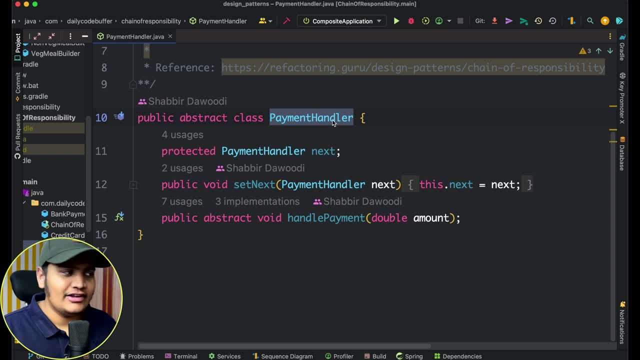 That is the payment handler. Okay, This is something we'll be able to handle our payment And within this payment handler, you can see that I have created one more property. That is the next payment handler. Okay, So you can see that I am having the property of the next handler. 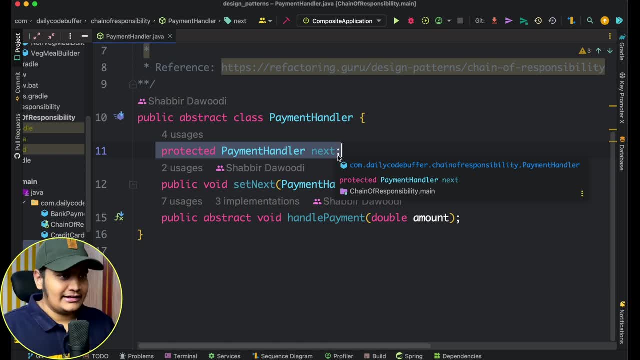 That is the next responsibility that it is going to do. Okay, And what's going to be my next handler? What is going to be my next responsibility to complete? Okay, So that two things I have added here and this is the method to add the next responsibility. 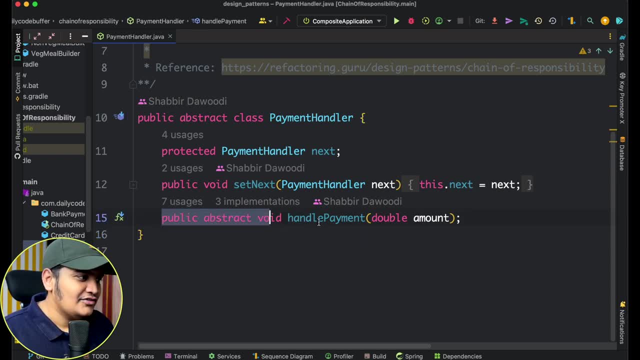 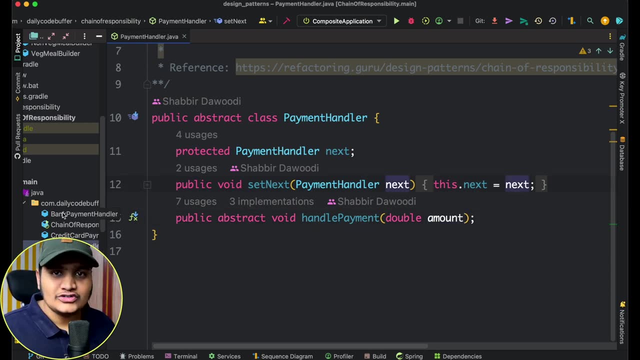 Simple thing, And now you can see. this is a method, abstract method, which is going to handle the payment, which will take the amount and which will handle the payment. This is something will be implemented by the concrete classes. Now let's go to the concrete classes. 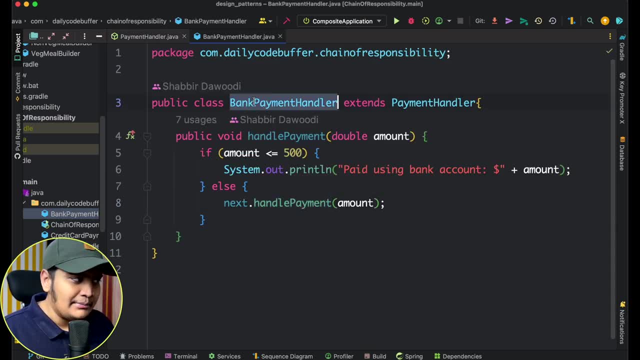 That is the bank payment handler. Okay, So this is a bank payment handler which is extending payment handler. Okay, And this has the handle payment method, which is taking the amount. And here you can see it's simple thing: If the amount is less than 500, okay. 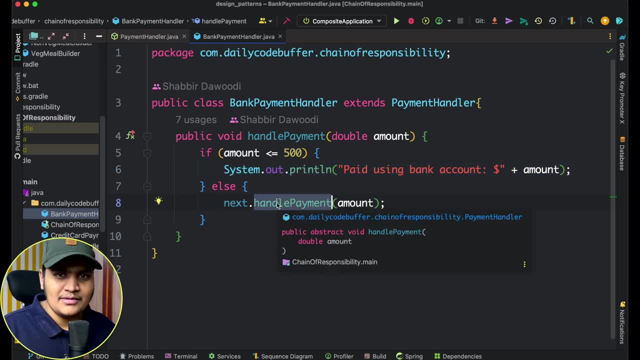 Process it Else. go to next dot. handle payment: Simple, Okay, If I'm able to handle it, that's good. I'm not able to handle it. Call the next responsibility: Okay, Simple. Same way. If I go to credit card, that's the same thing that I'm able to handle thousand rupees. 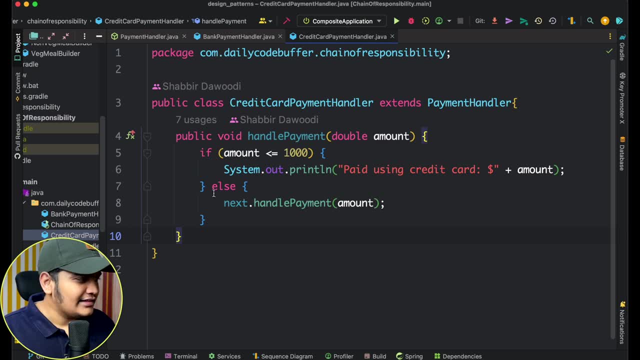 Okay, Thousand dollars, Whatever the currency is. If not, then go to the next handler. Same way for the people as well That I'm able to handle this, That's fine. Otherwise, go to the next handler So you can see that my all the handlers are ready. 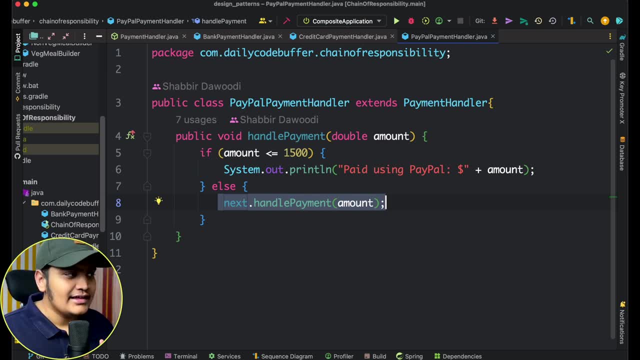 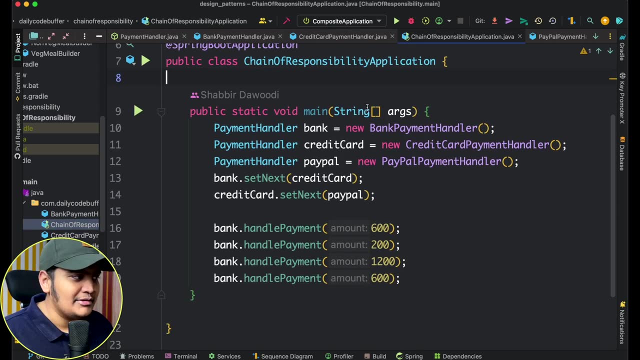 I have my base handler, that is, abstract class, and all the classes implementing this handle payment method. Okay, Now, this is my main method. That is the chain of responsibility application. This is my main method, And what I'm doing is I have created three payment handlers. 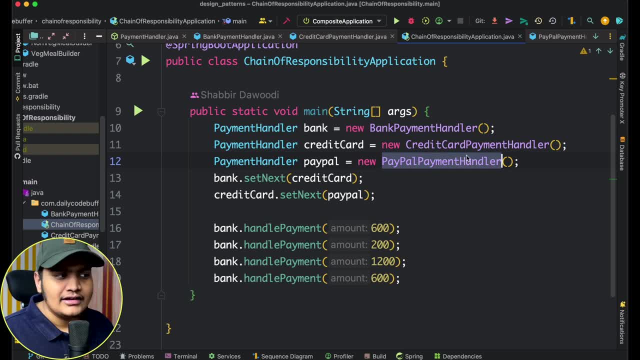 That is, bank payment handler, credit card payment handler and people, bank payment handler. And here you can see that I have added the responsibility that bank has the responsibility of credit card. It will give the responsibility to credit card. Credit card will give the responsibility to people. 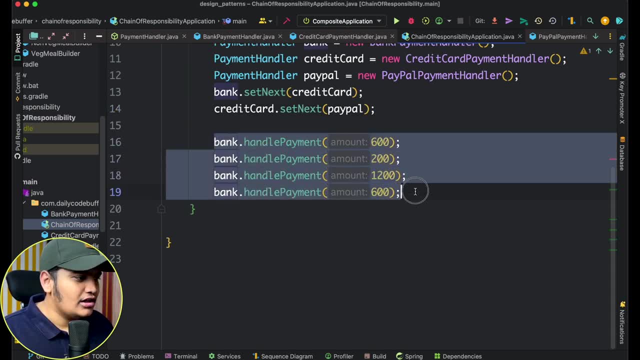 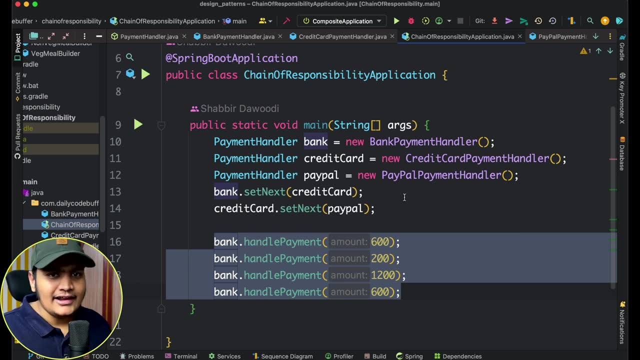 And now you can see that, with the bank, I am calling all these different methods Okay, Because your bank is your base handler, right? That's the starting point, So from there it will be able to traverse request throughout the all the responsibilities. 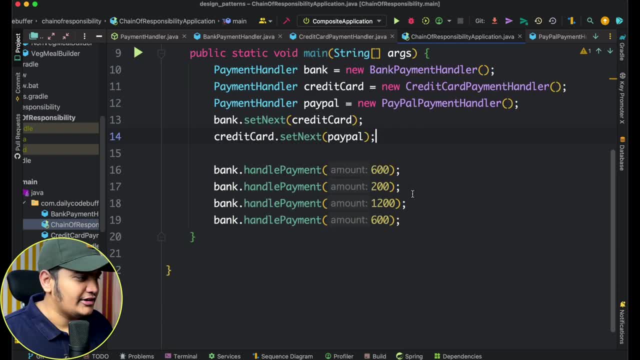 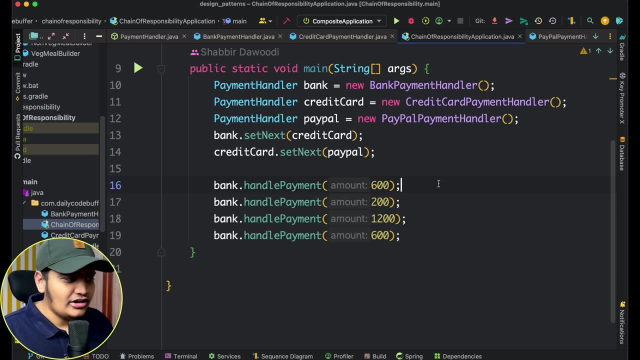 that you have given in the chain. So that's the idea about the chain of responsibility. Now we will go through this, all the different methods, and we will try to identify that which particular method will be called where. Okay, So we will go to $600 and $600. 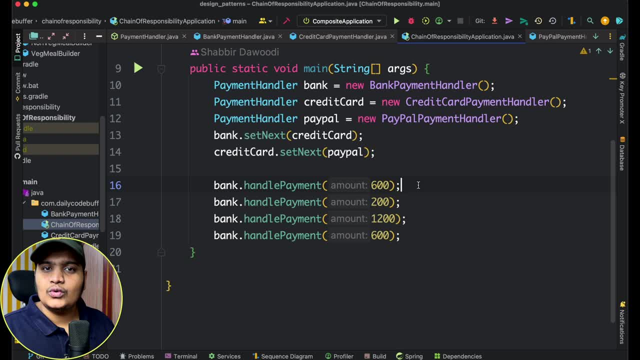 We will call bank handle payment method and bank can only handle 500, so it will be calling the next possible handler available. Okay, So the next possible handler we have added is credit card. Credit card can handle thousand, So it will be processed by credit card.